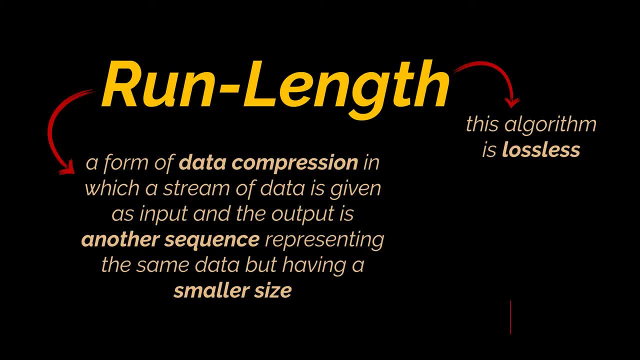 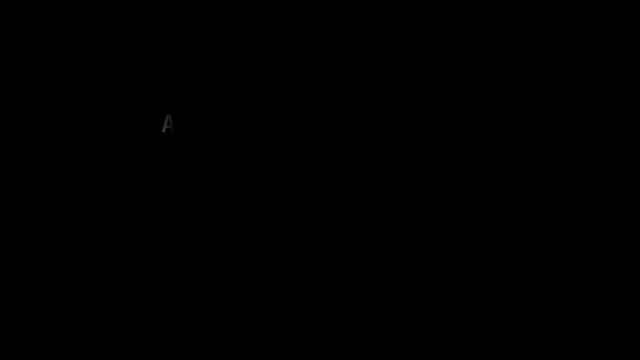 will be recovered when decoded and nothing will be lost. as compared to other compression algorithms, such as the LZW algorithm, which we will discuss in future videos, One of the most attractive features of this algorithm is its simplicity in both the encoding and the decoding. And to better visualize these functionalities, imagine you have this string of data as an 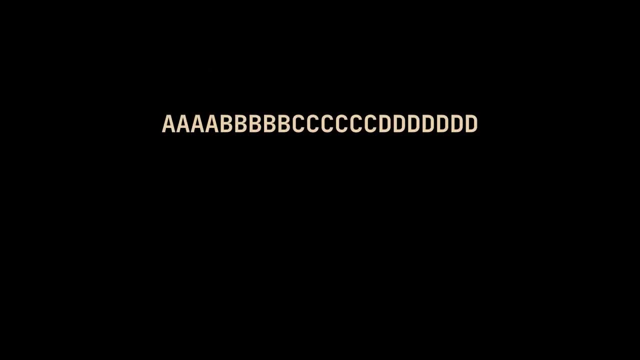 example, and suppose you want to encode it using the RLE algorithm. To do that you have to count the occurrences of each character inside this string, So the A is repeated four times, the B five times, and so on. Then you have to append every character alongside. 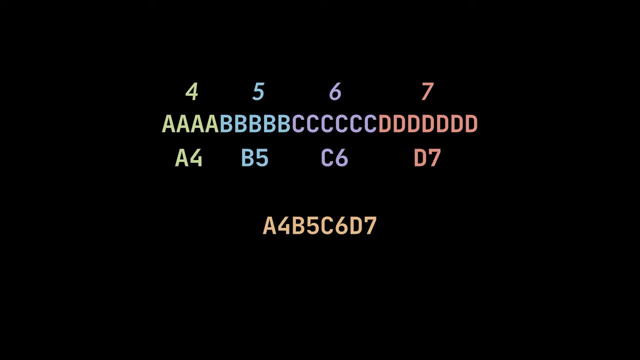 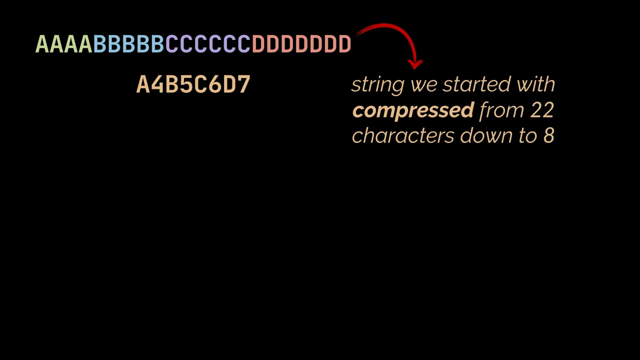 its number of occurrences. So the resulting compressed string we are going to obtain here is 25C6D7.. See, by counting the occurrences we were able to compress the string we started with from 22 characters down to just 8, which is 65% smaller. And this also means that the 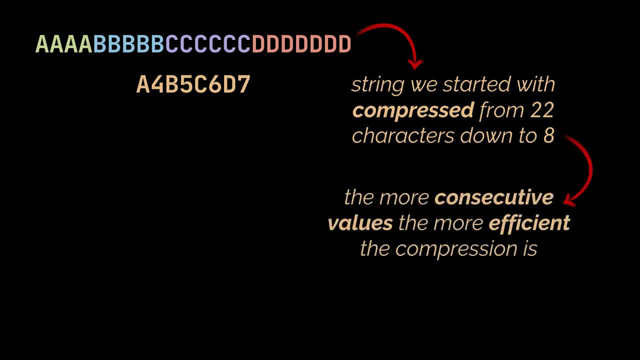 more consecutive values or characters in a row, the more space we save in the resulting compression. However, you may have noticed that this algorithm won't turn out to be useful on a sequence of data that frequently changes between values, such as the one you see in. 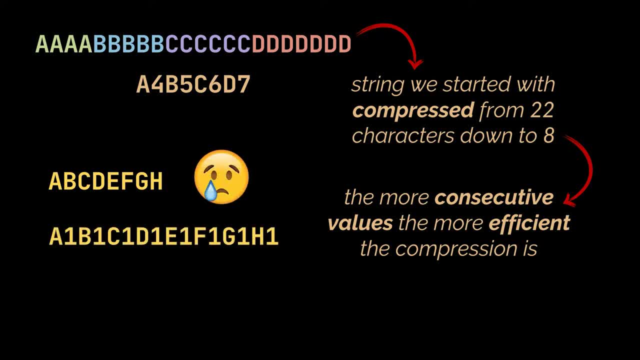 front of you. In fact, we could even increase the size of our data, since a single instance of a character results in two characters in the output of the encoding, ie an A becomes an A1.. Now, because of this, RLE is only good for certain types of data and applications. 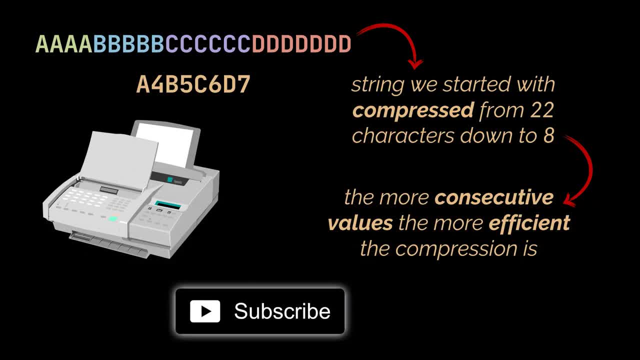 For example, fax machines and black and white pictures. both of these exclusively contain the bits 1 and 0. Therefore, the input is guaranteed to be made of runs of white pixels in the blank space and runs of black pixels within the text. 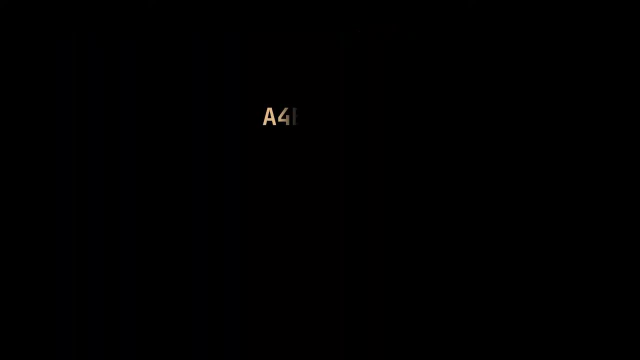 Finally, before kicking off the implementation, I want to briefly go over the decoding part, even though you most probably figured it out by now. So to decode or go back to our initial input, all we have to do is iterate over the generated string and try to extract the pairs. 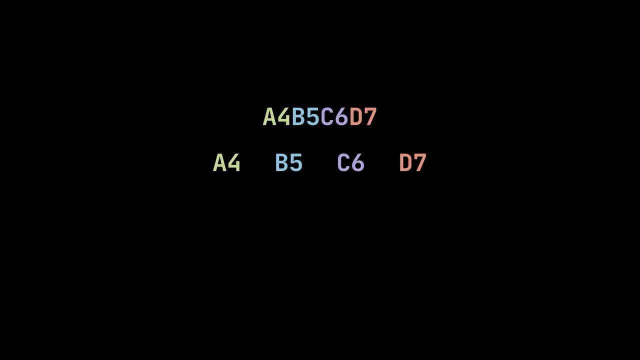 of character digits we created while encoding. After doing that, each character inside a pair should be appended as many times as the digit states to a newly created string, and the result will hopefully be the initial text we started with. So let's get started. 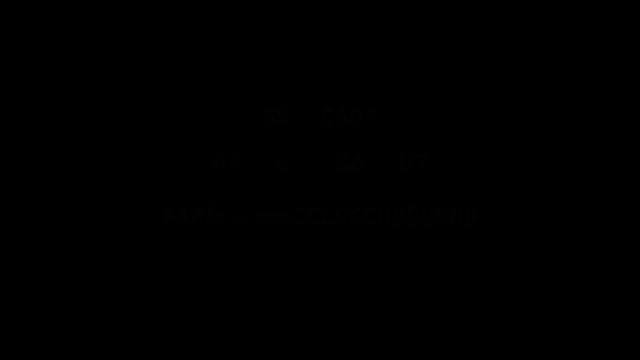 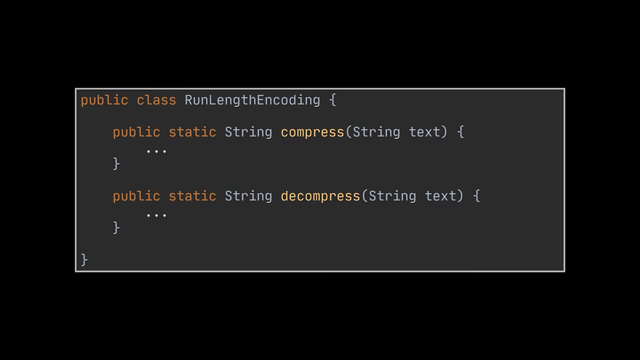 Let's get started. Okay, now that we know how RLE works and when it is used, let's tackle its implementation in Java. To do this, we are going to start by creating the runLengthEncoding class, and inside this class we'll have two methods: the compress and the decompress methods. Now, if you google, 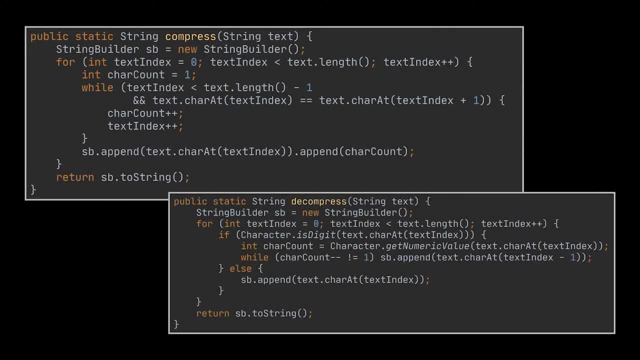 this algorithm. almost all the solutions you will find involve while loops that iterate over the characters of the input string and try to count the occurrences of consequent characters similar to the ones you see in front of you. So let's get started. 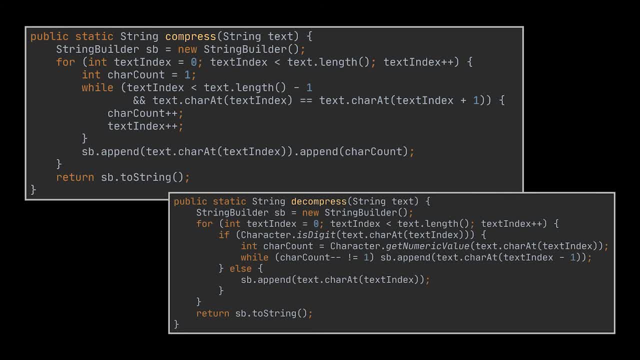 Let's start with the compress method, and we will use the compress method to create the pattern that is going to identify the character occurrences. for me, However, what I want to explain today is kind of an alternative and more generalized approach, even if the traditional one proved to be a bit faster. This approach involves the use 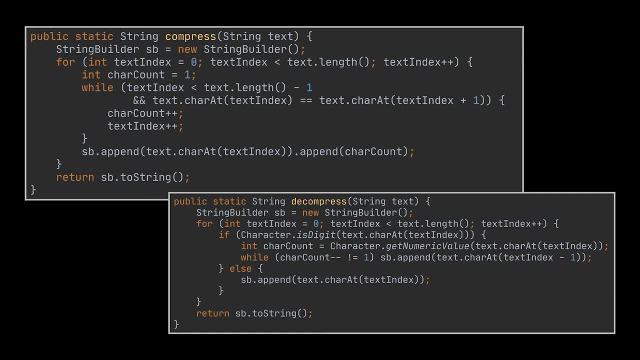 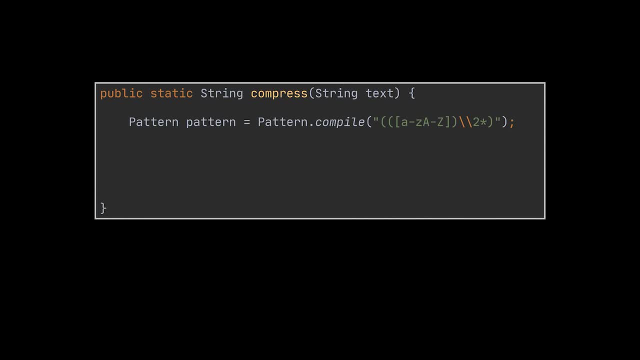 of regXs, and if you are not quite familiar with these, don't worry: we already have a video covering all you need to know about them. So, concerning the compress method, the first thing I am going to do is create the pattern. 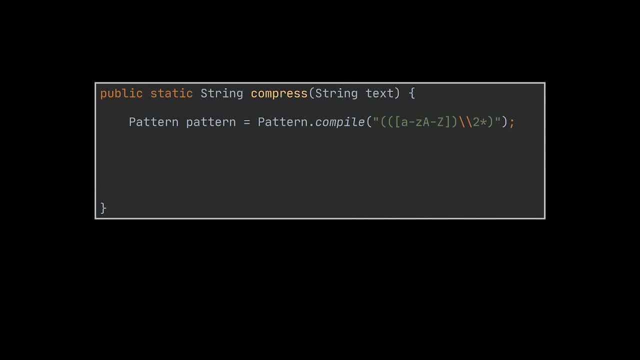 that is going to identify the character occurrences. for me, The first parenthesis defines the first group of the pattern. Therefore, the back center and the center are the first group of the pattern. Therefore, the back slash 2 represents the second pair of parenthesis. you see? 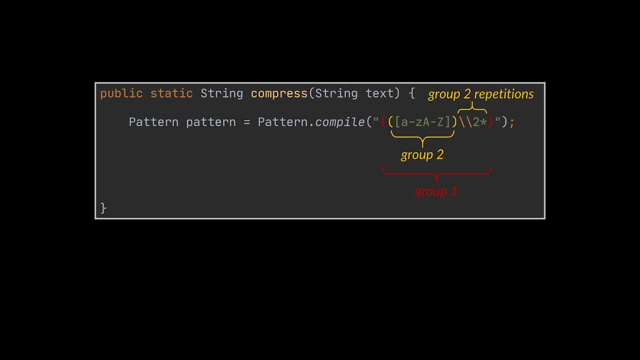 So what I am basically saying here is: I detect a character and then, because of the back slash 2 and the asterisk, I want to find all the consecutive occurrences of this same character. Take the same example we had at the beginning. If we apply this pattern on it, the resulting 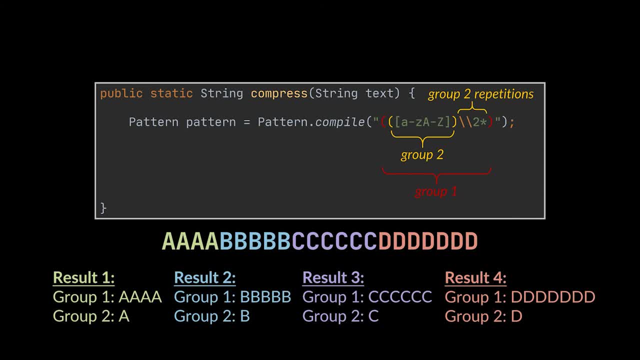 groups you are going to obtain are, as you can see, in front of you. So inside the first groups of our result sets we have the whole repeated block and inside the second groups we have the repeated character. Now that we know what this pattern does, we 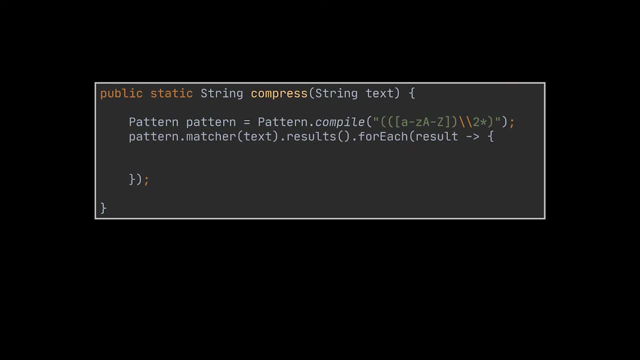 need to find matches for it in our input and loop over the results we found. What remains is generating the output string, and this string is made of each individual character, followed by the occurrences of this character. To do that, we have to create a